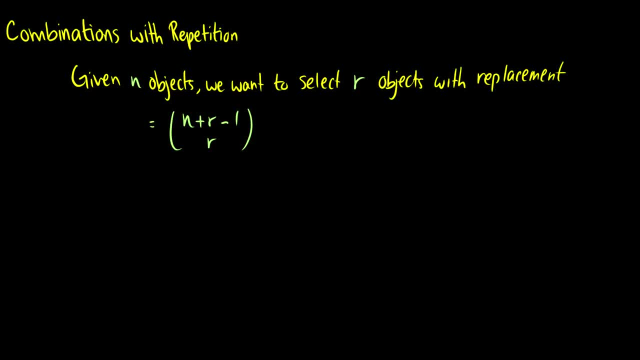 Welcome back to Discrete Mathematics. Today we're going to take a look at combinations with repetition. So we did combinations without repetition earlier, which was just n choose r. but in this case, when we have n objects and we want to select r of them with replacement, 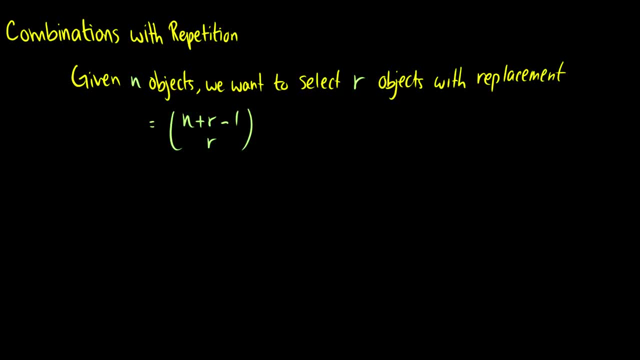 it's going to be n plus r minus 1- choose r. And I'm going to give you an intuitive explanation why. hopefully, and with the following example, I'll also give you another explanation intuitively, So you'll have two different angles to see this. So what we're going to do is we're going to take 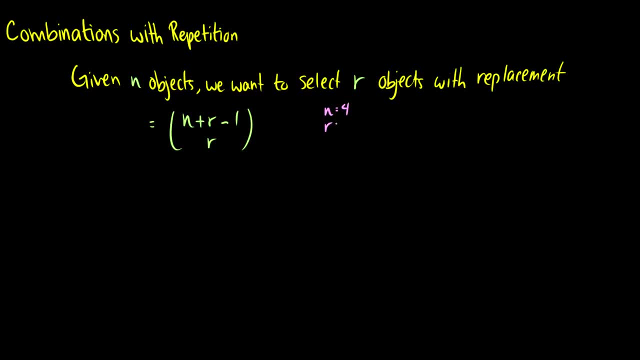 in our example, n is equal to 4 and r is equal to 3.. So we have four objects here. We're just going to call it 1, 2,, 3, and 4.. And what we're going to do is we're going to select. 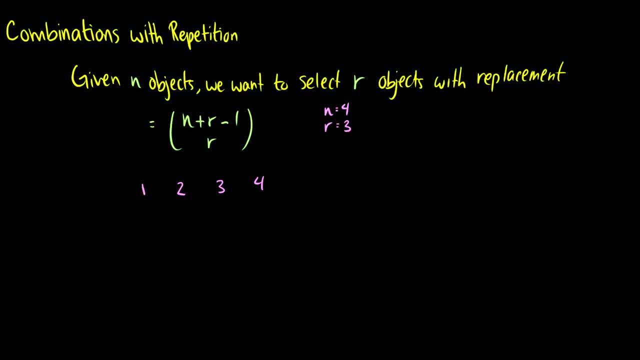 one of them. So for our first one we're selecting, we're going to take 2, and we're going to put 2 into a bin here. OK, so we selected 2.. So when we select things with combinations, we kind of cross it out and say, OK, we can't take this again. 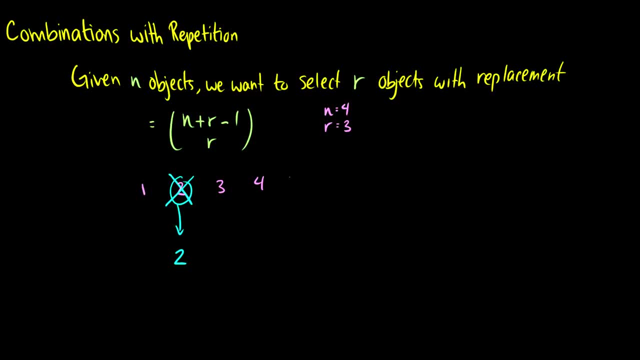 But we can take it again. so we have to add 2 back. OK, now, this time we take, let's take 4 next. So we put 4 in there. We're going to cross it out, But because we took 4 out, we have to add it back in because 4 gets. 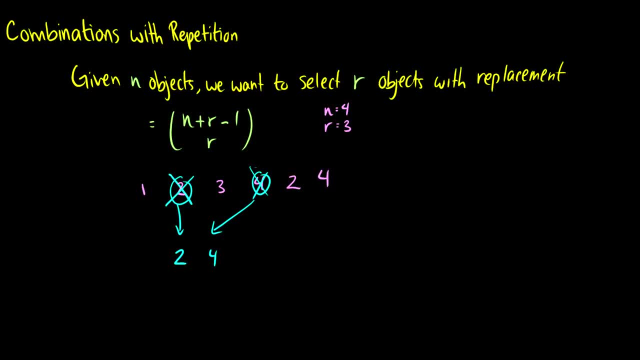 replaced. OK, so then let's take 4 again. So there we go. We selected 2,, 4, and 4.. So there we have it. We selected three objects from four, with repetition. So what we really did here is: out of five total objects, we chose three, So this is equal to 5,. 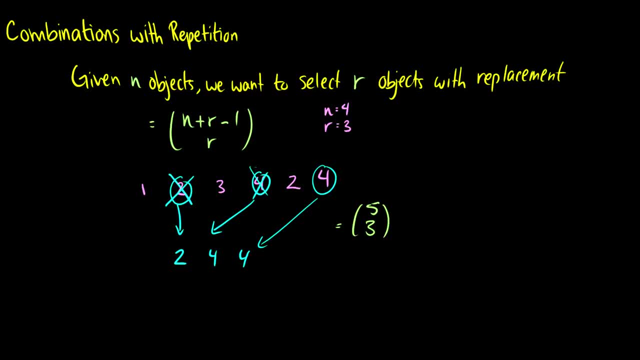 and we chose 3.. Now you're saying: hold on a second, but if I take one first and this 2 right here becomes a 1 instead, it's a different set, Not necessarily. The intuition here is that you're just replacing and you're filling in an empty spot. for whatever, the first one you chose is. 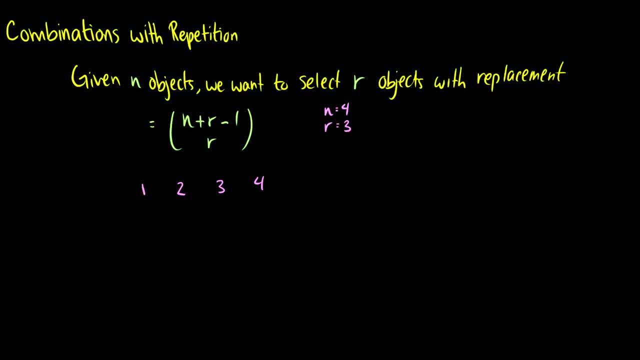 one of them. So for our first one we're selecting, we're going to take 2, and we're going to put 2 into a bin here. OK, so we selected 2.. So when we select things with combinations, we kind of cross it out and say, OK, we can't take this again. 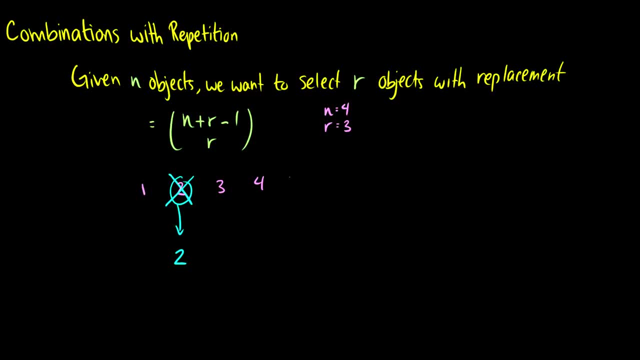 But we can take it again. so we have to add 2 back. OK, now, this time we take, let's take 4 next. So we put 4 in there. We're going to cross it out, But because we took 4 out, we have to add it back in because 4 gets. 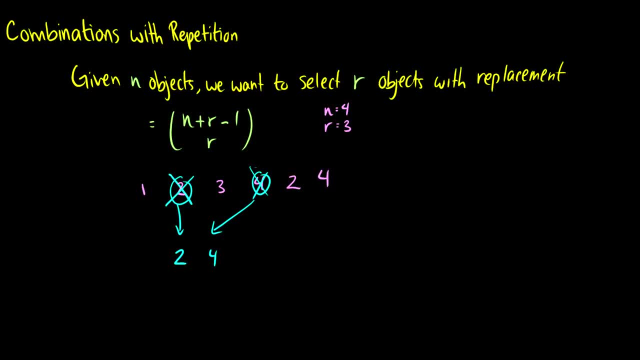 replaced. OK, so then let's take 4 again. So there we go. We selected 2,, 4, and 4.. So there we have it. We selected three objects from four, with repetition. So what we really did here is: out of five total objects, we chose three, So this is equal to 5,. 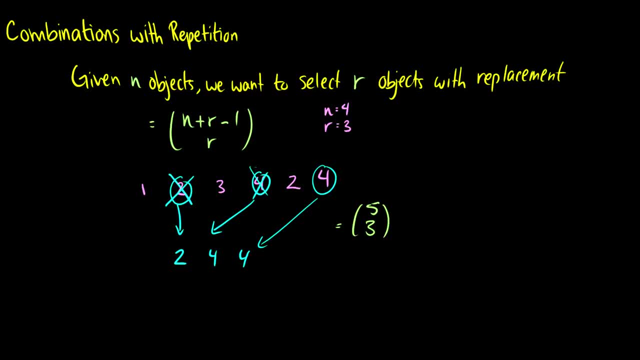 and we chose 3.. Now you're saying: hold on a second, but if I take one first and this 2 right here becomes a 1 instead, it's a different set, Not necessarily. The intuition here is that you're just replacing and you're filling in an empty spot. for whatever, the first one you chose is. 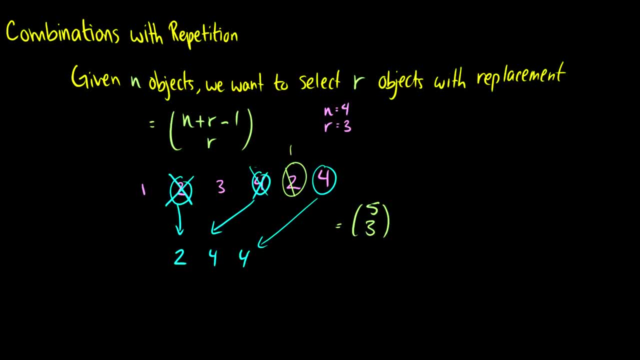 and then you're filling an empty spot for whatever the second is. And, of course, when we choose the third one, we don't have to add a new slot, because we're done What we're doing here. so you can see that this is 5, choose 3.. If we put in our sorry, 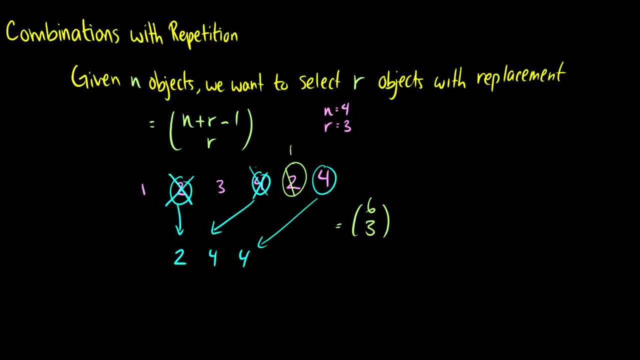 this should be 6 choose 3.. If we plug in our formula here, we would get 4 plus 3 minus 1 choose 3, which is just equal to 6 choose 3.. So that's the intuition here. Now, what can we do? 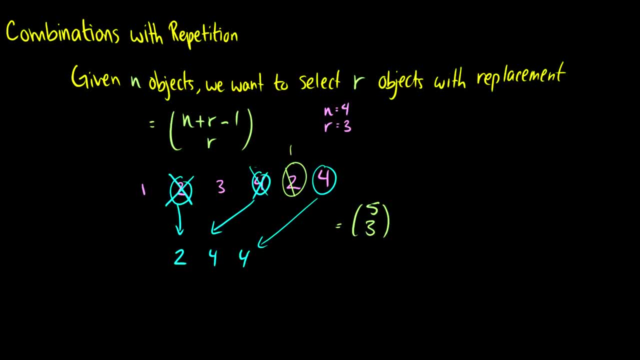 and then you're filling an empty spot for whatever the second is. And, of course, when we choose the third one, we don't have to add a new slot, because we're done What we're doing here. so you can see that this is 5, choose 3.. If we put in our sorry, 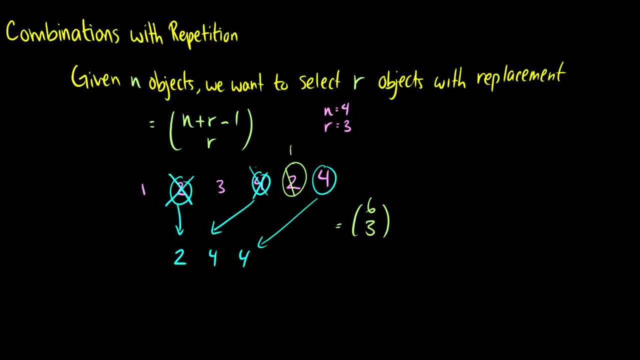 this should be 6 choose 3.. If we plug in our formula here, we would get 4 plus 3 minus 1 choose 3, which is just equal to 6 choose 3.. So that's the intuition here. Now, what can we do? 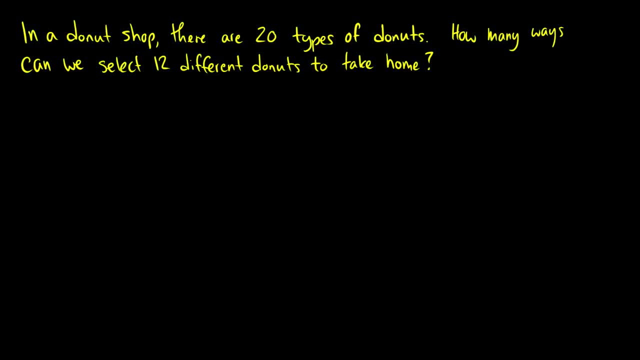 Well, we can say, OK, suppose we have a doughnut shop with 20 different kinds of doughnuts. So you know, you have chocolate glazed chocolate, the Boston cream, There's tons of different donuts, but we want to select 12 different doughnuts to take home. So really what we're doing here. 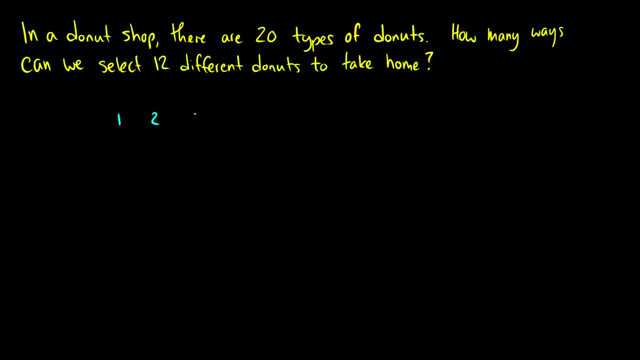 is we're listing out. Okay, we have type 1.. We have type 2.. We have type 3, all the way up to type 19 and type 20.. We do the same thing as before. We say, okay, I want type 2, so we put 2 in our bin. 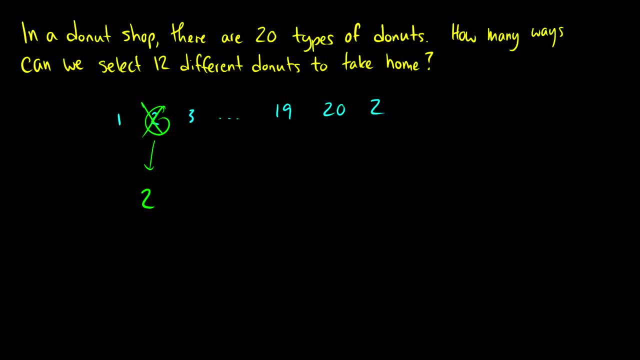 cross it out and then we add an extra slot for 2 so we can take it again. So we have: n is equal to 20,. we have r is equal to 12, because we want 12 different donuts. so we get 20 plus 12 minus 1. 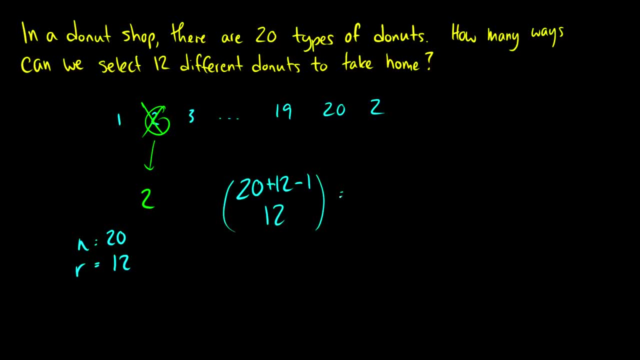 choose 12,, which is just equal to 31: choose 12.. So that's one way of looking at these types of problems. Another way is this way where we say: okay, x1 plus x2 plus x3 is equal to 7, all of. 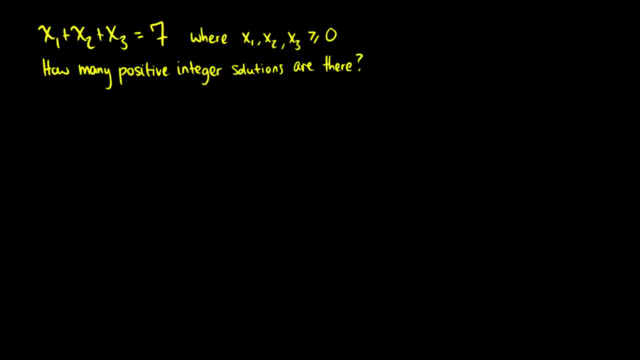 these are greater or equal to 0.. How many positive integer solutions are there to this equation? So what we have this time is we have three different bins, and we're going to call them x1,, x2, and x3. And we want to put 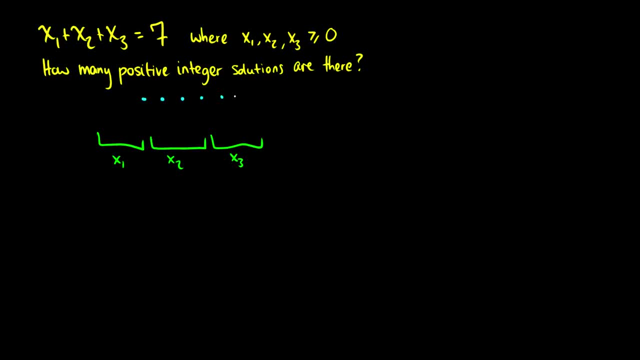 seven objects into these bins, So we could put this one there, that one there. we're going to fill x2 up with those two and x3 we'll get in these three, So this will be: 2 plus 2 plus 3 is equal to 0.. And we're going to put 7 objects into these bins, So we're going to put 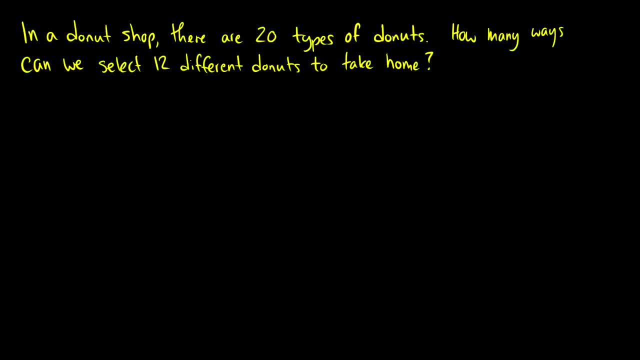 Well we can say: OK, suppose have a donut shop with 20 different kinds of donuts, So you have chocolate glazed chocolate, Boston cream. there's tons of different donuts, But we want to select 12 different donuts to. 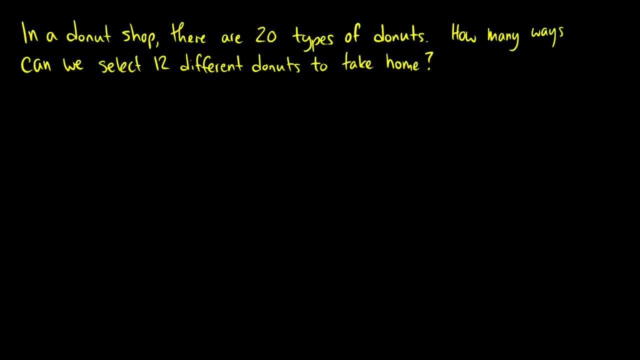 take home. So really, what we're doing here is we're listing out: OK, we have type 1, we have type 2, we have type 3, all the way up to type 19 and type 20.. We do the same thing as before. We say, OK, I want type 2, so we put 2 in our bin. 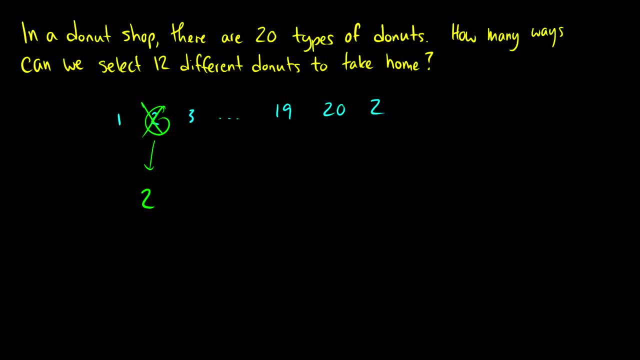 cross it out and then we add an extra slot for 2 so we can take it again. So we have: n is equal to 20,. we have r is equal to 12, because we want 12 different donuts. so we get 20 plus 12 minus 1. 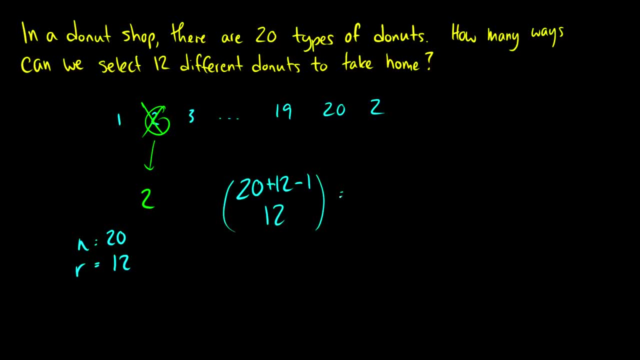 choose 12,, which is just equal to 31: choose 12.. So that's one way of looking at these types of problems. Another way is this way where we say: okay, x1 plus x2 plus x3 is equal to 7, all of. 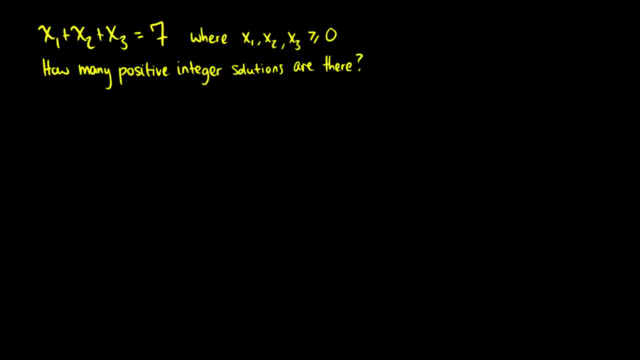 these are greater or equal to 0.. How many positive integer solutions are there to this equation? So what we have this time is we have three different bins, and we're going to call them x1,, x2, and x3. And we want to put 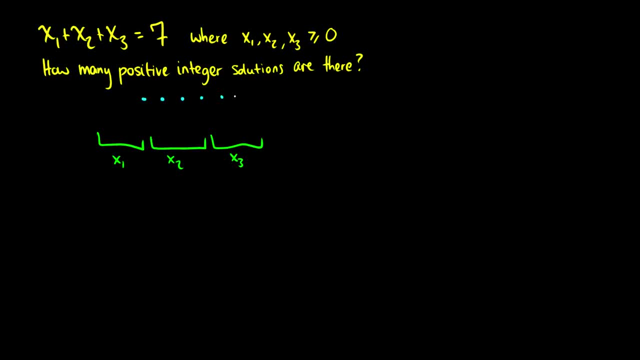 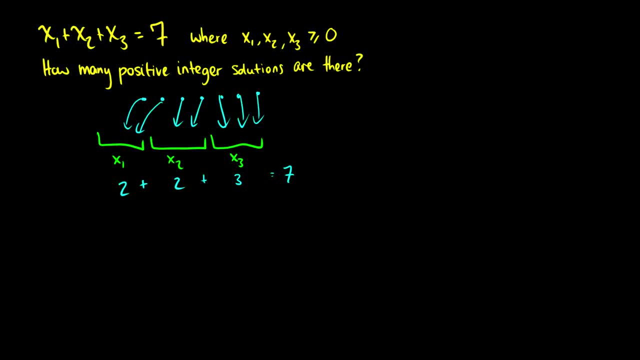 So you're saying: okay, wait, why isn't this just 3 times 3 times 3 times 3?? So it would be 3 to the 7, because each circle has a way of going into seven different containers. Well, that's permutations. 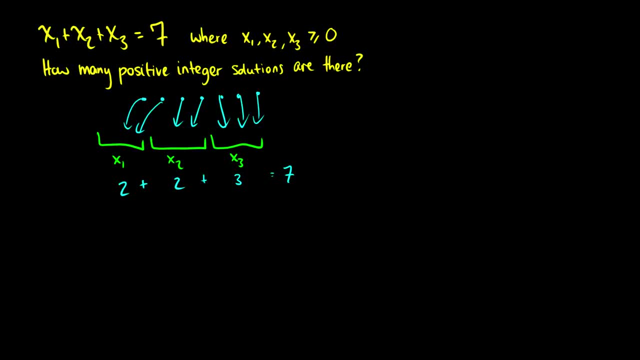 for one And all of these integers. they're indistinguishable, which means they're all identical. So you remember the multinomial theorem where we have, like north and east and we have to divide by the amount of east factorial and n factorial. It's the same idea. So instead, what we're going to do is introduce this other 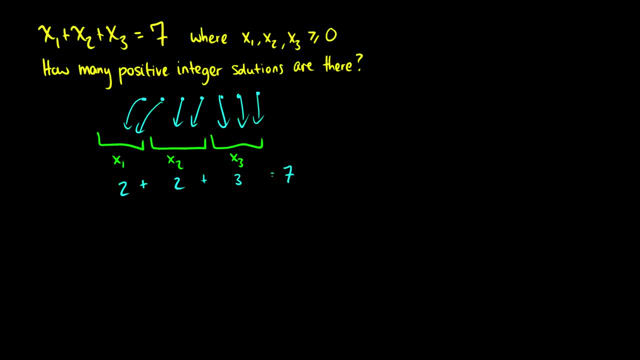 x1 and x2, and x3 is equal to 7.. So you're saying, Okay, why isn't this just 3 times 3 times 3 times 3?? So it would be three to the seven, because each circle has and has a way of going into seven. 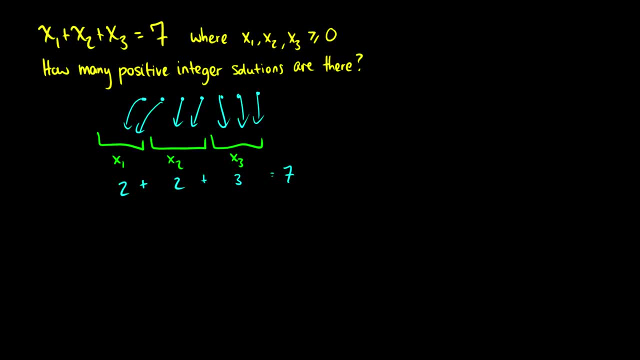 different containers. Well, that's permutations for one And all of these integers there, indistinguishable, which means they're all identical. So you remember the multinomial theorem where we have, like, norths and easts and we have to divide by the amount of east factorial and n factorial. 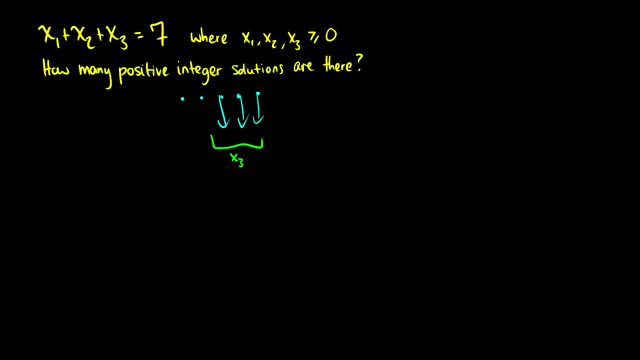 It's the same idea. So instead, what we're going to do is introduce this other intuitive notion of: okay, here's seven objects: 3,, 4,, 5,, 6,, 7, and I want three bins. 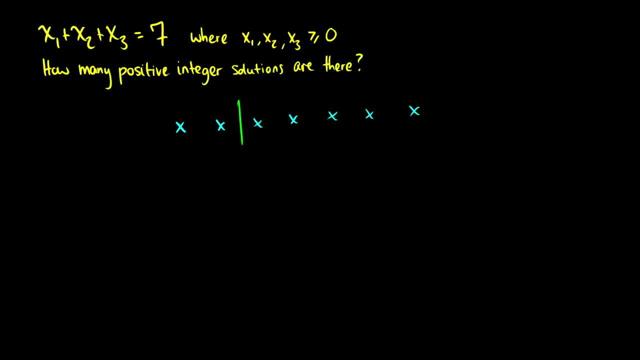 So to make three bins, all I need to do is insert two lines anywhere. So in this case we have x1,, x2, and x3.. So x1 has 2,, x2 has 3, and x3 has 2.. 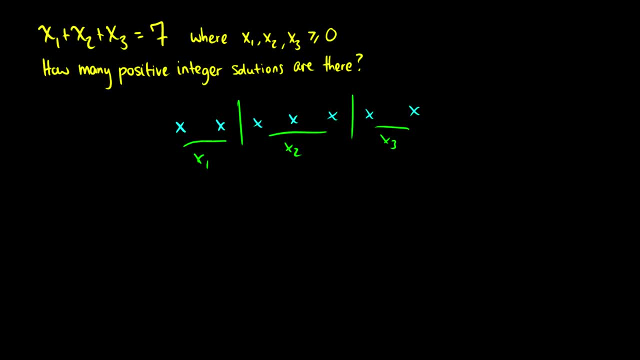 Okay, that's not bad. So what if we want one of the bins to have 0? Then we just put this line here. So this is x0, and sorry, this should be x1. And this bin, x3, can be here. 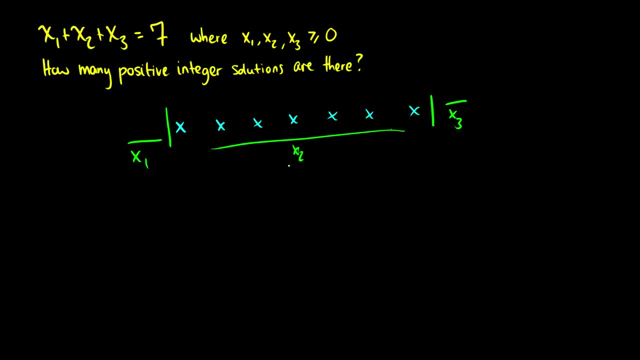 And then x2 can have all 7.. So that's also a possibility. So what are we really doing here? Well, really, we're taking. how many dividers do we need To get three bins? we need two dividers. 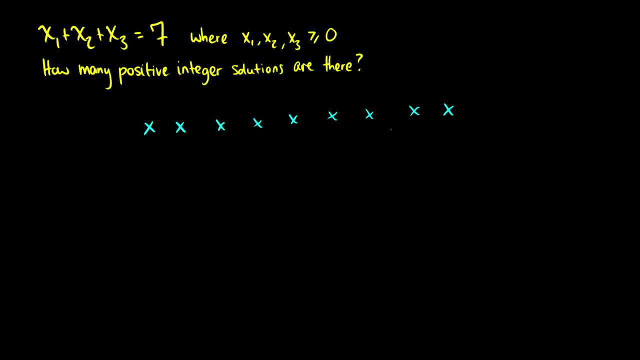 So we're actually working with eight different spots- Sorry, nine different spots- And then we just put our dividers into two of those spots. So this is 1 plus 4 plus 2.. Or we can put our dividers in these two spots. 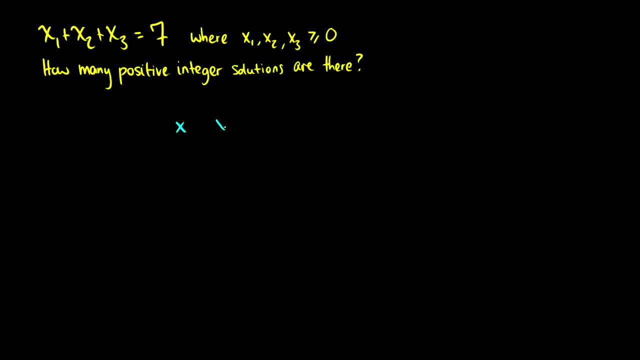 intuitive notion of: okay, here's seven objects: 3,, 4,, 5,, 6,, 7.. And I want three bins. So to make three bins, all I need to do is insert two lines anywhere. So instead of 3 bins, I'm going to insert 2 lines anywhere. 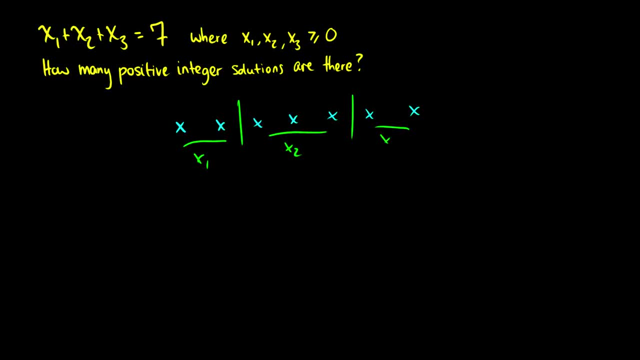 So instead of 3 bins, I'm going to insert 2 lines anywhere. So instead of 3 bins, I'm going to insert 2 lines anywhere. In this case, we have x1,, x2, and x3. So x1 has 2,, x2 has 3, and x3 has 2.. Okay, that's not bad. 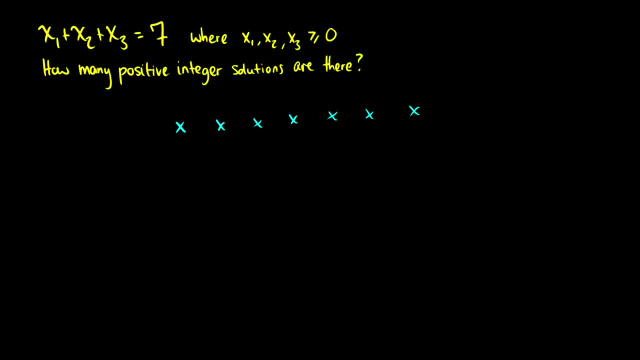 So what if we want one of the bins to have 0? Then we just put this line here. So this is x0. And sorry, this should be x1. And this bin x3 can be here And then x2 can have all 7.. 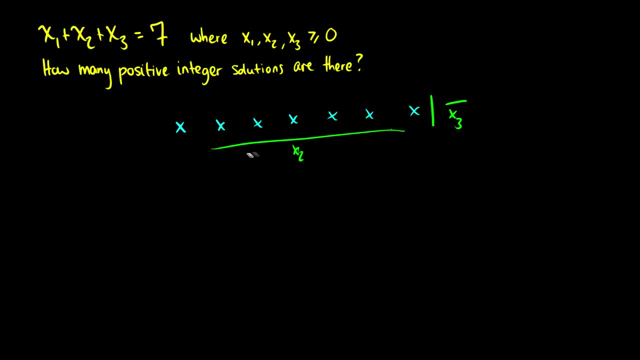 So that's also a possibility. So what are we really doing here? Well, really, we're taking: how many dividers do we need To get three bins? we need two dividers, So we're actually working with eight different spots- Sorry, nine different spots- And then we just put our dividers into two. 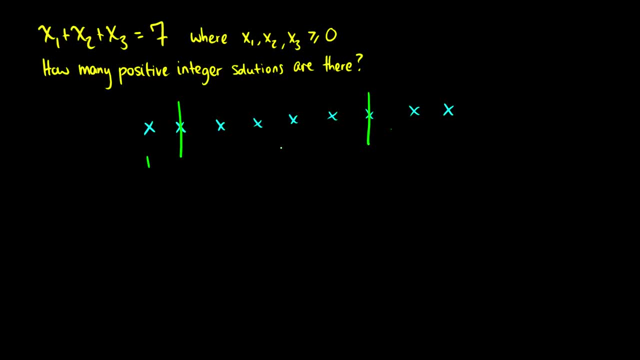 of those spots. So this is 1, plus 4, plus 2.. Or we can put 2, plus 4, plus 2. And then we can put our dividers in these two spots And this is just 7, plus 0, plus 0. So you take the amount of. 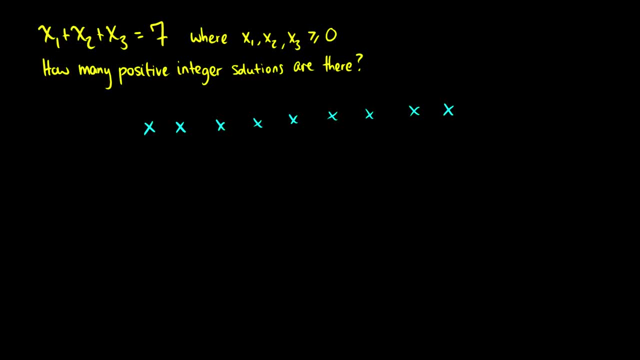 dividers you need, which is going to be n minus 1.. And then you just put them in the extra n minus 1 slots you've added. So for this equation, if we take n plus r minus 1, we're going to have 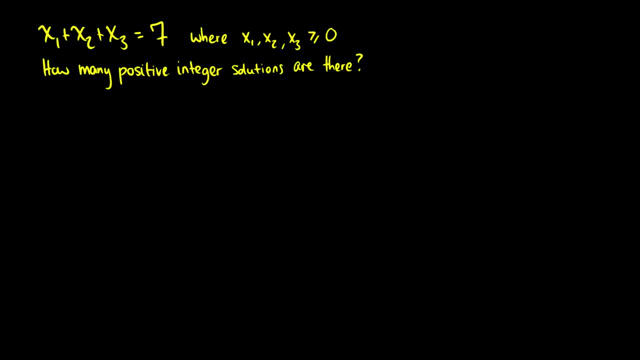 1, choose r. It's a good idea first to tell us more generally which ones are n and which ones are r. So the general solution is that x1 plus x2, all the way up to xn, is equal to r. We'll have. 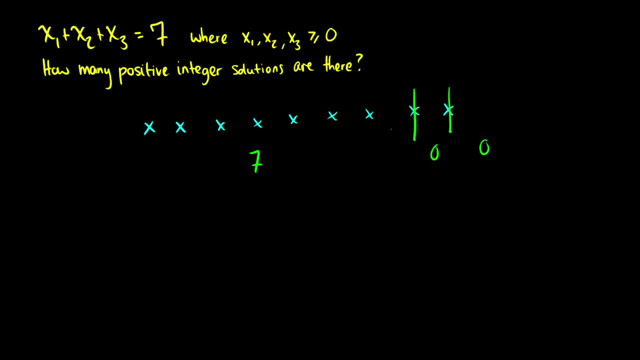 And this is just 7 plus 0 plus 0.. So you take the amount of dividers you need, which is going to be n minus 1. And then you just put them in the extra n minus 1 slots you added. 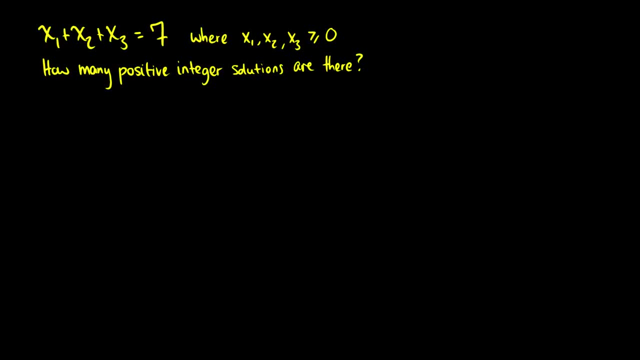 So for this equation, if we take n plus r minus 1, choose r. it's a good idea first to tell us more generally which ones are n and which ones are r. So the general solution is that x1 plus x2, all the way up to xn, is equal to r. 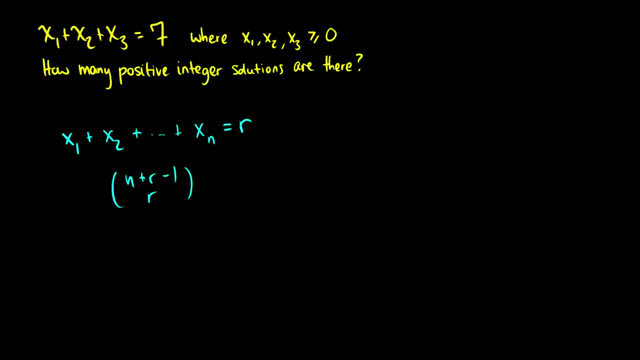 We'll have n plus r minus 1 choose r solutions where all of the x's are greater or equal to 0. So, in this case specifically, we just have 3 plus 7 minus 1 choose 7 solutions, which is equal to 9- choose 7,. 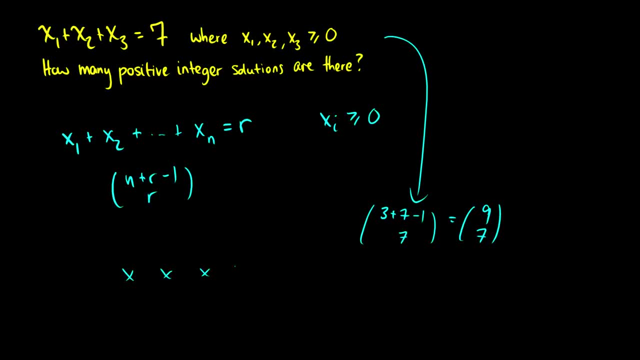 which is the same thing as saying: okay, I have 7 objects here, but I need two dividers. So I'm going to add two more options And I'm going to pick two of them to be dividers. So we know that this is equal to 9. choose 2 by the symmetry property. 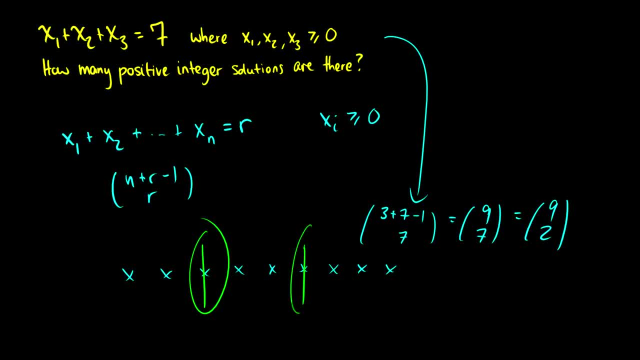 So this is the same way as saying: okay, I just chose two of my 9 objects to be dividers, So that's the difference here. All right, let's do something a little bit more challenging. that wasn't in the first time I did this video. 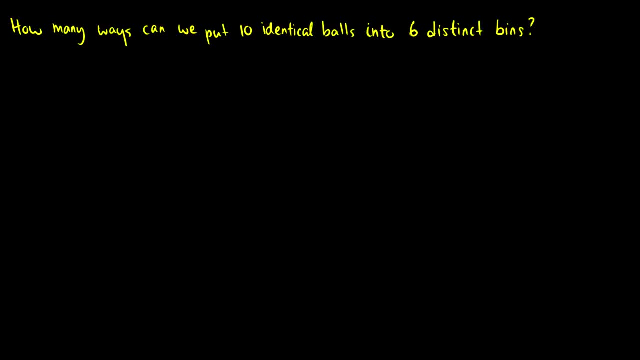 Right after this quick example here with the word problem, how many ways can we put 10 identical balls into 6 distinct bins? Well, this is the same thing as saying that x1 plus x2, all the way up to x6, is equal to 10, because this right here is the total balls. 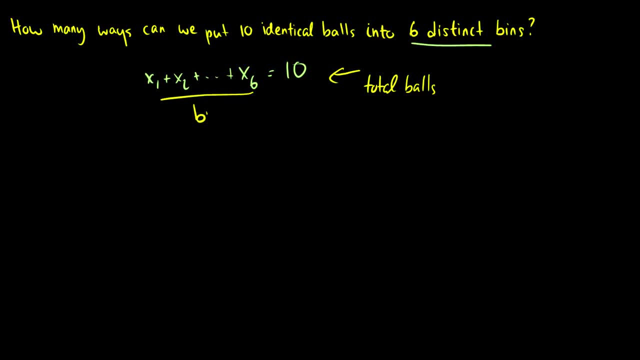 which is like the total numbers And this right here are the bins, 6 distinct bins. So this is just 6 plus 10 minus 1 choose 10, which is just equal to 15 choose 10.. Or 15 choose 5, because we need 5 dividers. 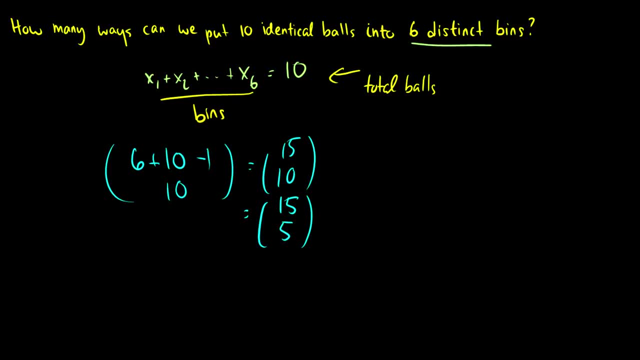 to get 6 different bins. So that was a word problem. I rushed through that a little bit, but it follows the exact same argument as before. So here's: something I didn't do in the original video was when one of our conditions has to be greater than another number. 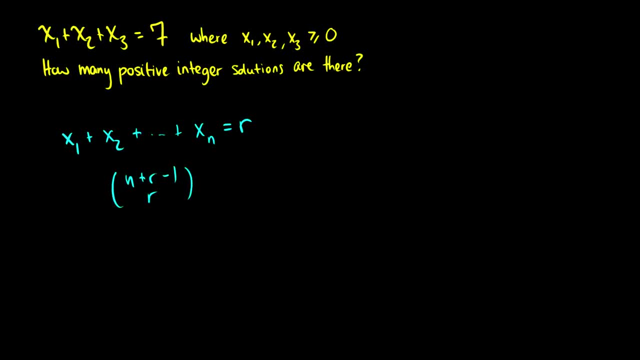 n plus r minus 1. choose r solutions where all of the x's are greater or equal to 0. So in this case specifically, we just have 3 plus 7 minus 1, choose 7 solutions which is equal to 9, choose 7.. Which is the same thing as saying, OK, I have. 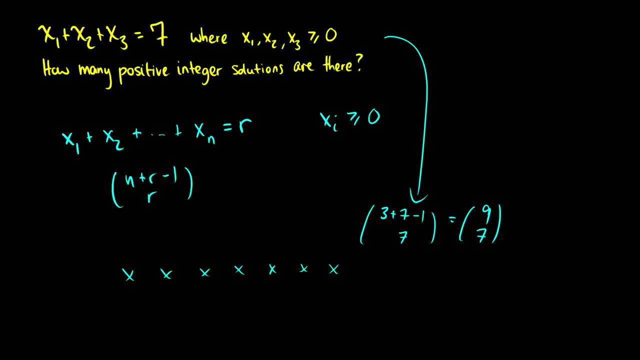 7 objects here, but I need 2 dividers. So I'm going to add 2 more options And I'm going to pick 2 of them to be dividers. So we know that this is equal to 9. choose 2 by the symmetry. 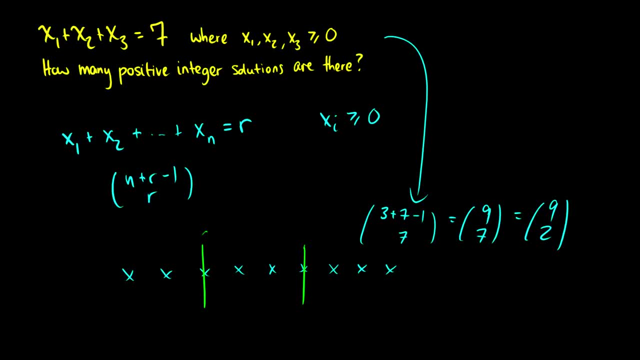 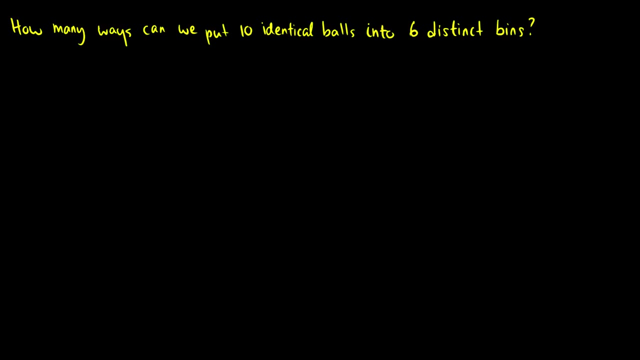 property. So this is the same way as saying: OK, I just chose 2 of my 9 objects to be dividers, So that's the difference here. All right, let's do something a little bit more challenging. that wasn't in the first time. I did this video Right after this quick example here with the word: 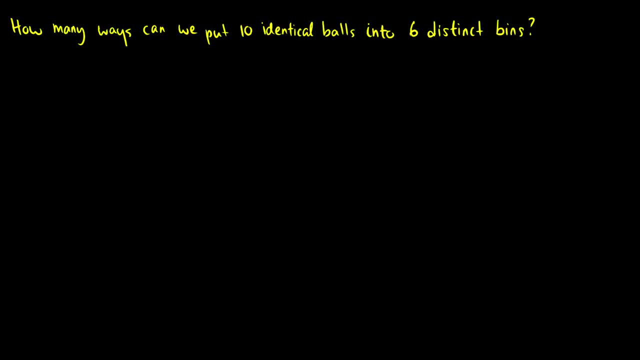 problem: how many ways can we put 10 identical balls into 6 distinct bins? Well, this is the same thing as saying that x1 plus x2, all the way up to x6, is equal to 10, because this right here is the total balls, which is like the total numbers, And this right here are the bins 6. 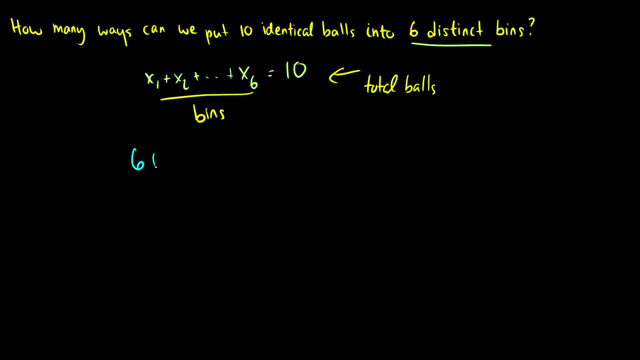 distinct bins. So this is just 6 plus 10 minus 1 choose 10,, which is just equal to 15 choose 10.. Or 15 choose 5,, because we need 5 dividers to get 6 different bins. So that was a word problem. 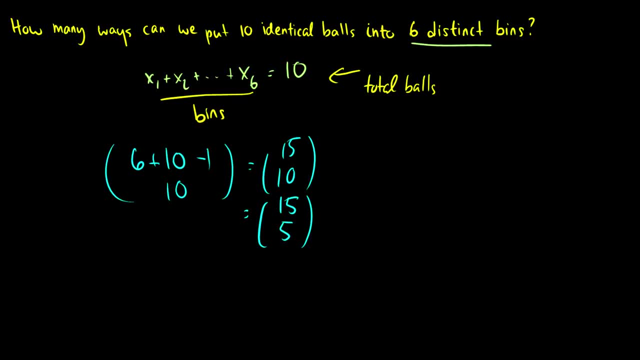 I rushed through that a little bit, But it follows the exact same argument as before. So here's something I didn't do in the original video was when one of our conditions has to be greater than another number, So x3 has to be. 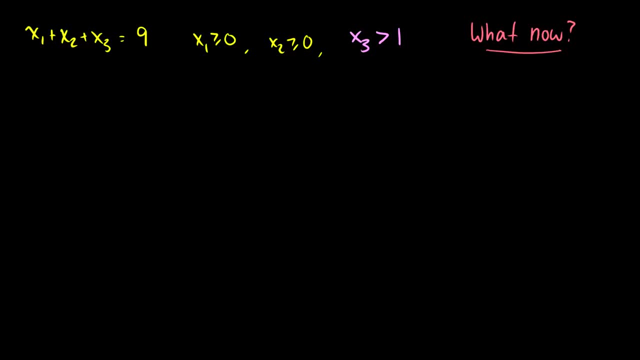 greater than 1.. So what this really means is that x3 has to be greater than or equal to 2.. So these are the same thing I'm saying: it has to be greater than 1, so it can be greater or equal to 2.. OK, 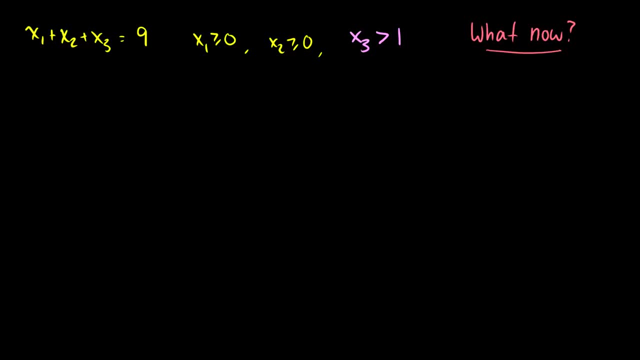 So x3 has to be greater than 1.. So what this really means is that x3 has to be greater than or equal to 2.. So these are the same thing I'm saying. it has to be greater than 1, so it can be greater or equal to 2.. 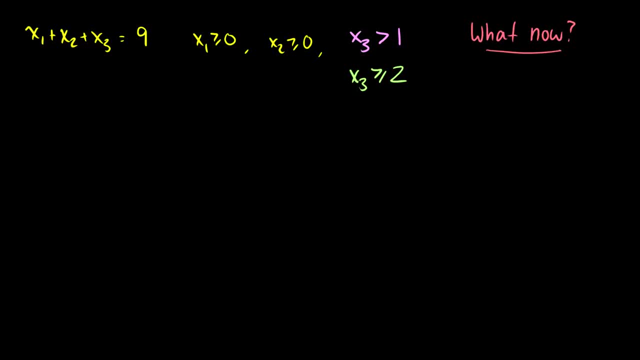 Okay. So let's start out here and say: let's convert this to a different type of problem. Let's, instead of having objects in a row, let's make shelves of objects. So we have a shelf x1,, a shelf x2, and a shelf x3.. 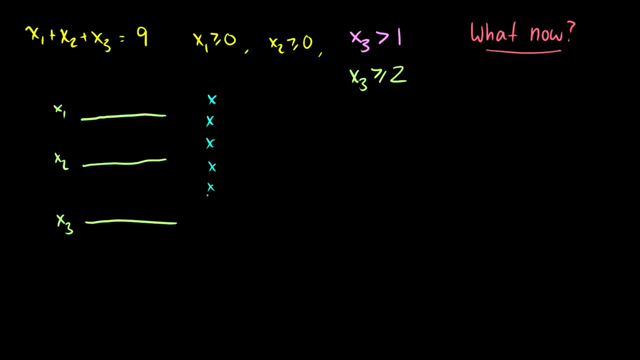 And I have 9 objects to put on these shelves. In fact, let's just say they're books, So these are going to be our books. So the shelf 3 has to have at least 2 books. So we're going to put 2 books on the shelf. 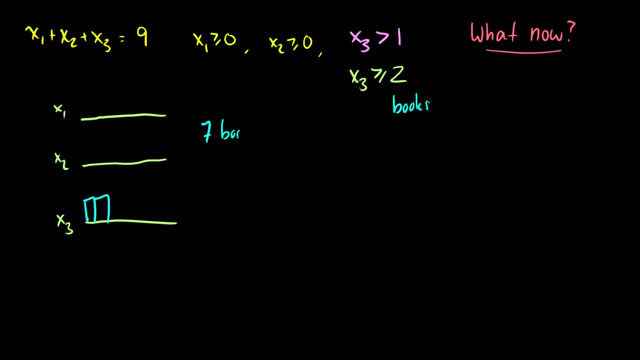 So what do we have left? Well, we now have 7 books left to distribute between these 3 shelves. So really, this problem right here is actually just x1 plus x2.. Plus x3 is equal to 7, where all of our x's are greater than 0,. 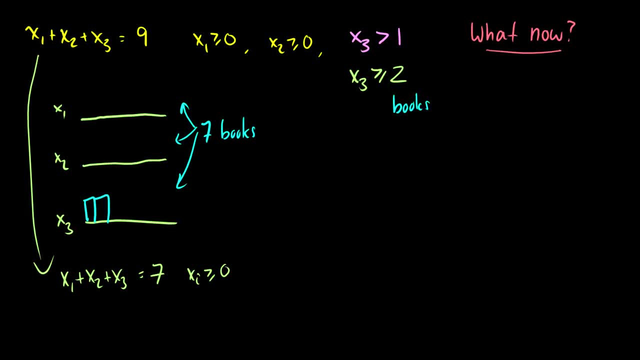 greater or equal to 0, which we know is just the same thing as 9 to 7 from the previous example. So here's the question: Well, how do we do that algebraically? So let's do this algebraically here. 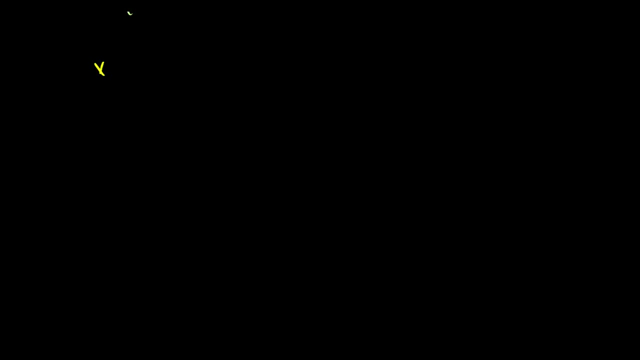 I'm just going to copy the question: x1 plus x2 plus x3.. So we're going to say x1 is equal to 9 where x3 is greater than or equal to 2.. Okay, what we're going to do is make a substitution. 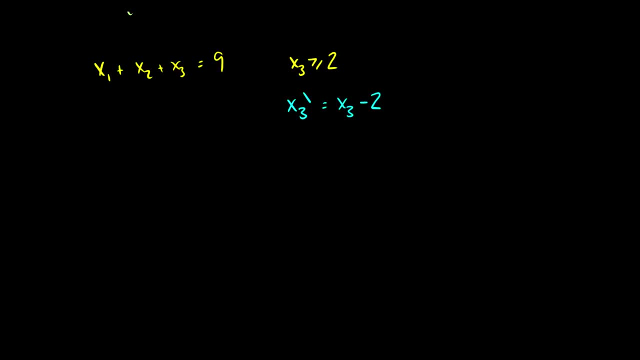 We're going to say x3 prime is equal to x3 minus 2.. So that way, x3 prime is going to be greater or equal to 0. So what we get is we get x1 plus x2 plus. well, hold on, we have to substitute x3 in. 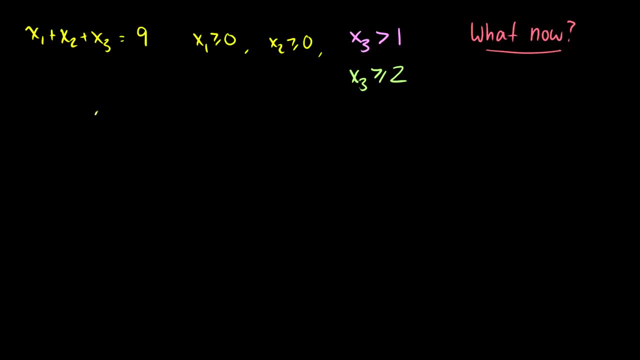 OK. So let's start out here and say: let's convert this to a different type of problem. Let's, instead of having objects in a row, let's make shelves of objects. So we have a shelf x1, a shelf x2, and a. 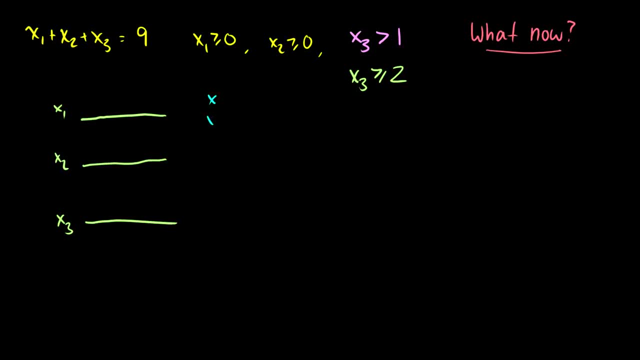 shelf x3. And I have 9 objects to put on these shelves. In fact, let's just say they're books, So these are going to be our books. So the shelf 3 has to have at least 2 books, So we're going to put 2 books on the shelf. So what do we have left? 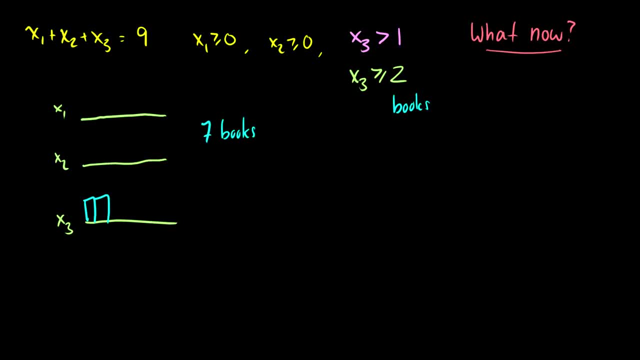 Well, we now have 7 books left to distribute between these 3 shelves. So really, this problem right here is actually just: x1 plus x2 plus x3 is equal to 7.. Where all of our x's are greater than 0, greater or equal to 0,, which we know is just the same thing as 9,, 2,, 7 from the previous example. 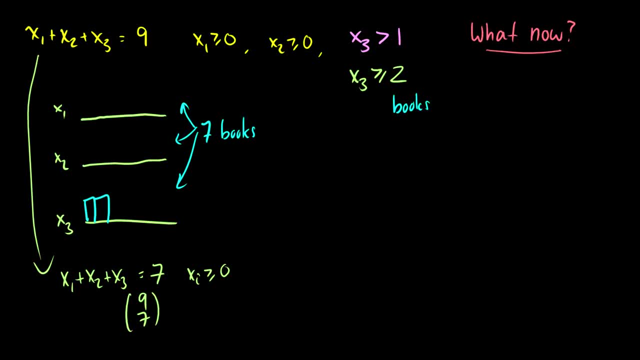 So here's the question: Well, how do we do that algebraically? So let's do this algebraically here. I'm just going to copy the question: x1 plus x2 plus x3 is equal to 9, where x3 is greater than or equal to 2.. 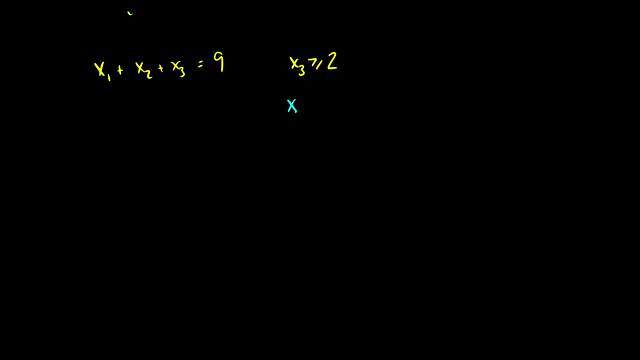 Okay, what we're going to do is make a substitution. We're going to say x3 prime is equal to x3 minus 2, so that way x3 prime is going to be greater or equal to 0. So what we get is we get x1 plus x2 plus. well, hold on, we have to substitute x3 in, So x3 is the same thing as x3 prime plus 2.. 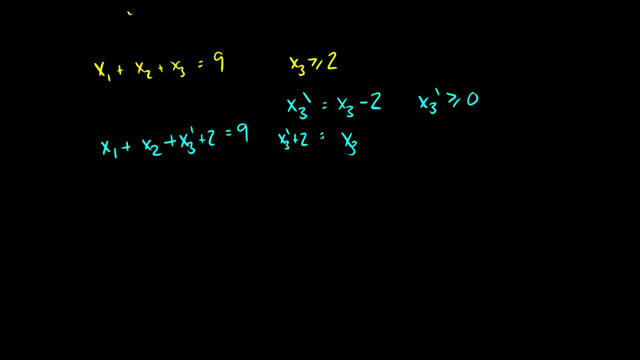 x3 prime plus 2 is equal to 9.. So we just substitute it in: x3 prime plus 2 equals 9, because we want to shift this 2 here to a 0. So we made the substitution possible And now we just use some algebra here.